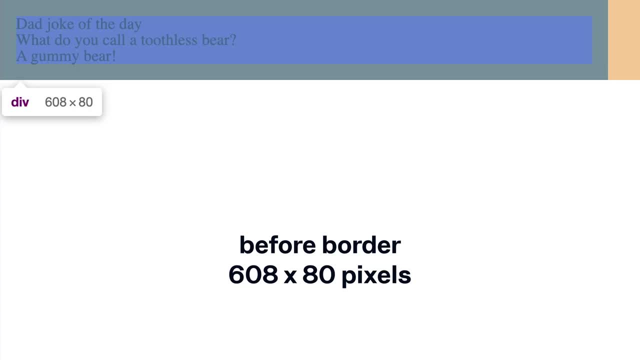 to the divider. I can also add a border to the divider. I can also add a border to the divider. The important concept to remember with borders is that they add to the total width and height of the element, even when the height and width are explicitly defined. 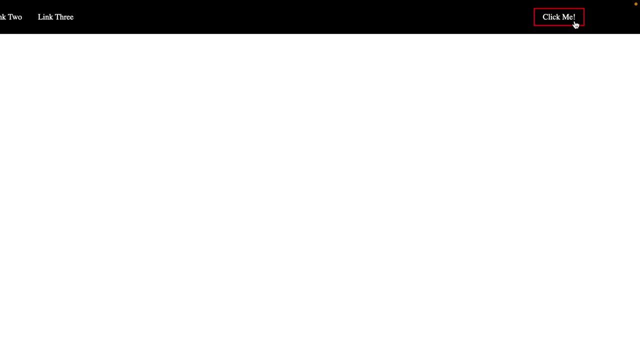 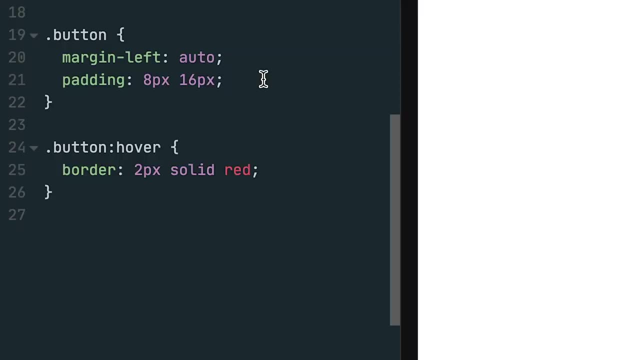 To help show how this works. let's say we have a button on a page that we want to add a border to. when a user hovers over it, You'll notice that the content shifts once I hover over the button. But why is this? The button doesn't have a border in its default style, so hovering 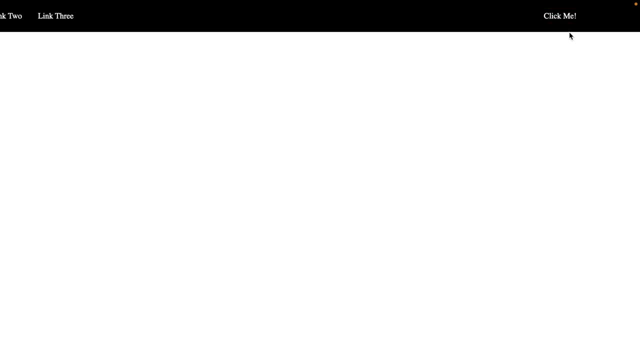 over the button increases its size, pushing the rest of the elements away. To fix this issue, I'll add the same border to the button's default style, but will change the color to transparent. Now, when I hover over the button, the content doesn't shift. 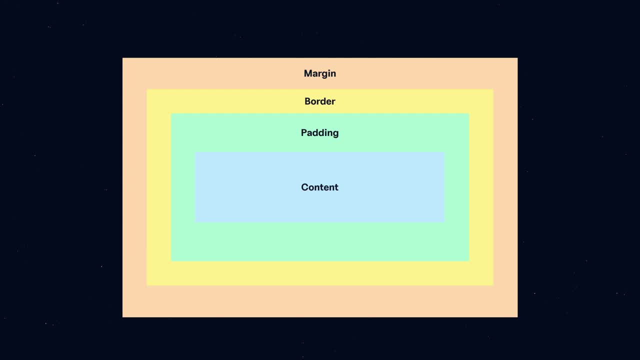 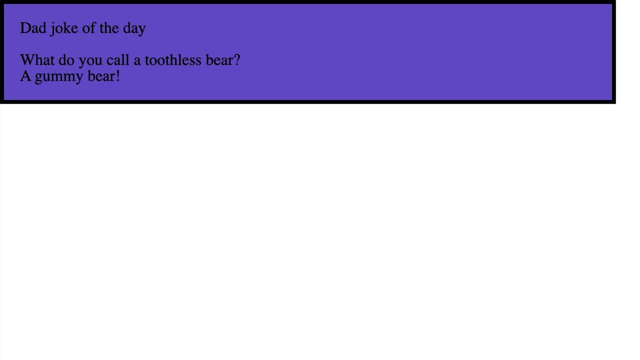 The last concept is margin, which clears an area outside the border. In our example, I'll add a bottom margin of 16 pixels to the heading tag and 8 pixels to the paragraph tags. The catch with margins is that they can sometimes behave unexpectedly because of margin collapse. 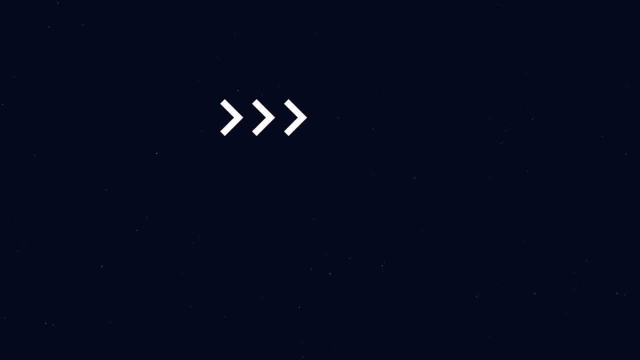 Watch this video here to learn more about that. And now that you know how spacing works on the web, go out and build some beautiful boxes. 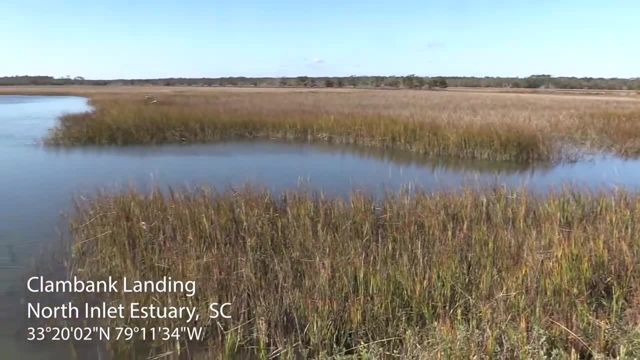 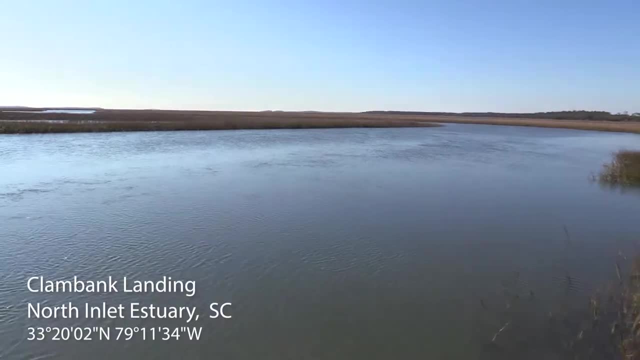 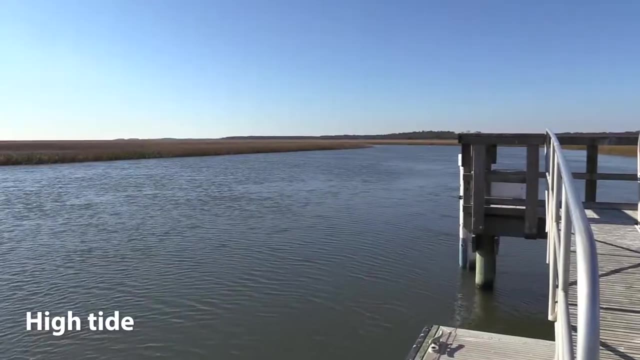 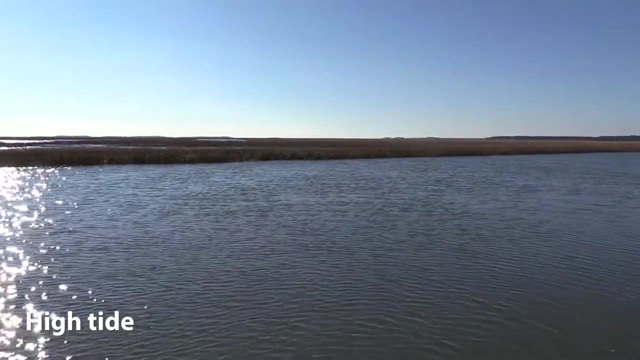 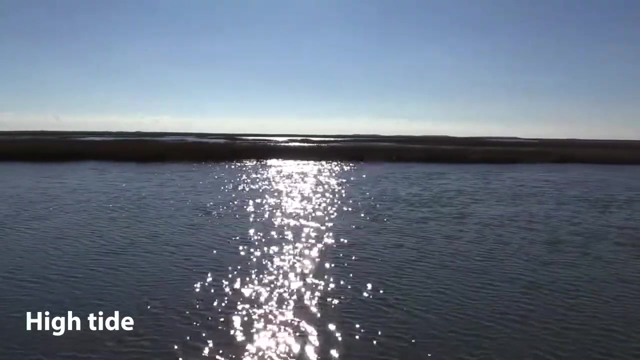 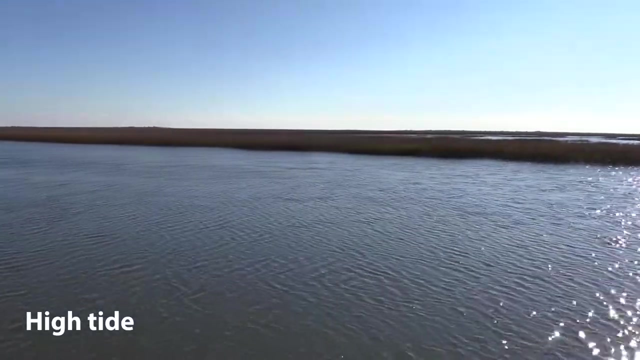 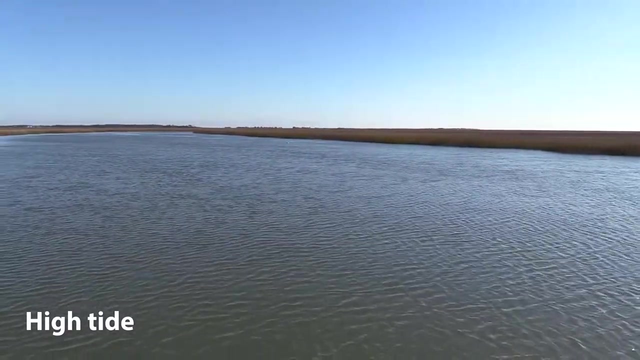 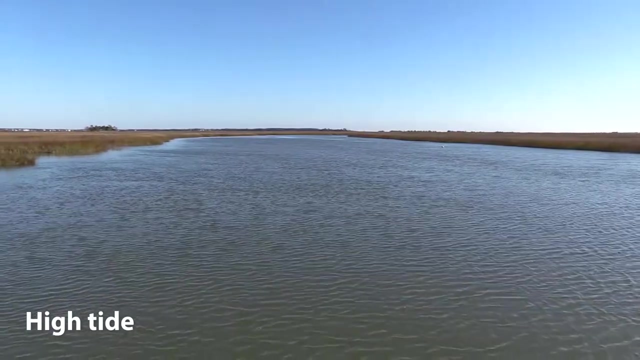 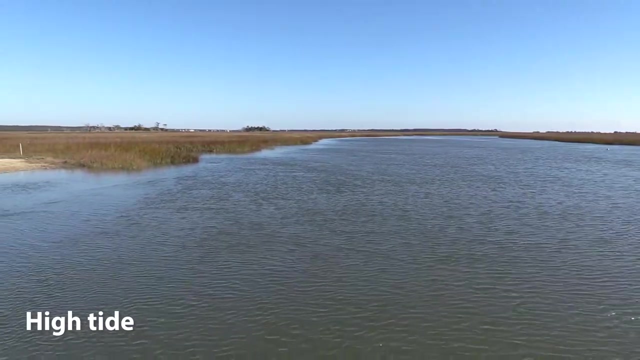 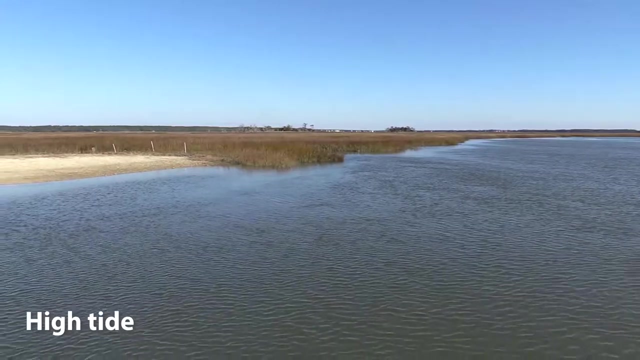 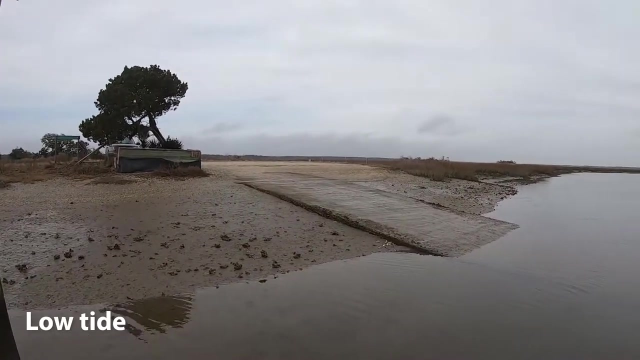 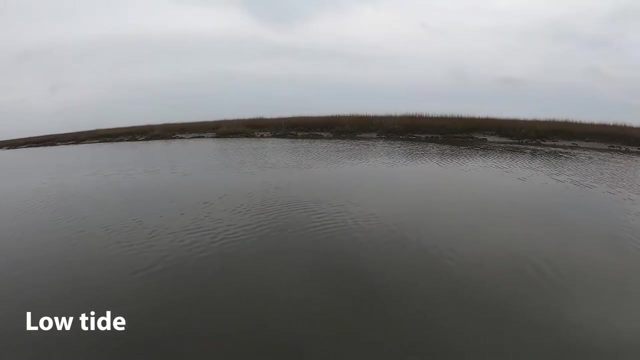 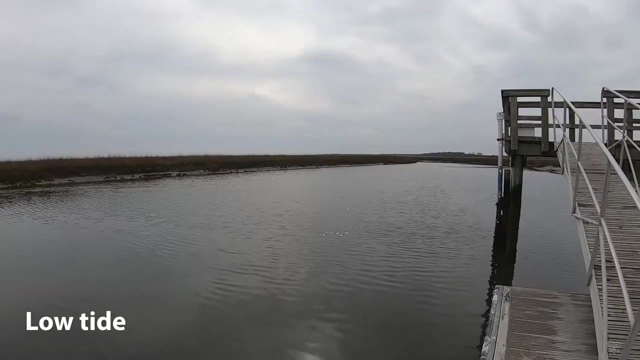